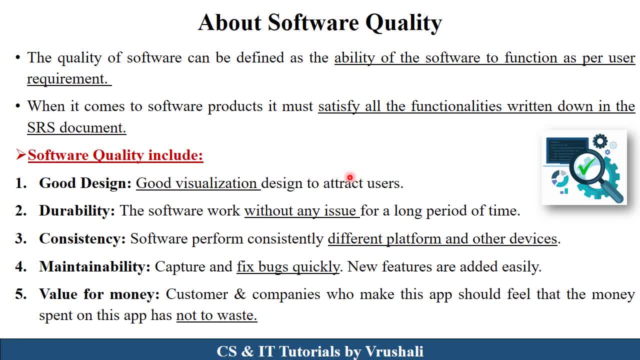 software also having some other words like a good design: means your software have provided a good visualization and good user interface, with multiple user attracted towards your website and application. Next one is a durability- long period of time. the next one is a consistency: means your software can perform consistently. 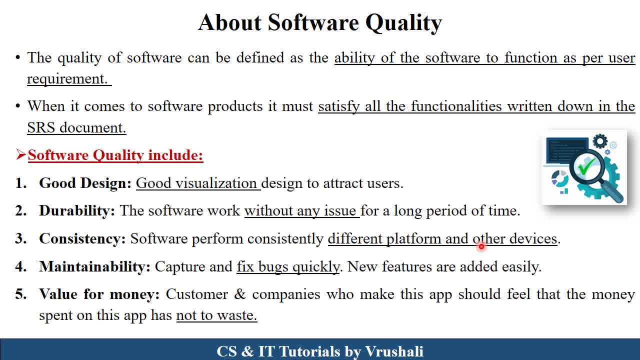 on different platform devices and different versions of operating system. next one is a maintainability means if any errors have occurred, in particular software, that can be solved easily or you can also add new features in your product easily. this is called as maintainability. and the last one is a value for money: means a company would develop a particular 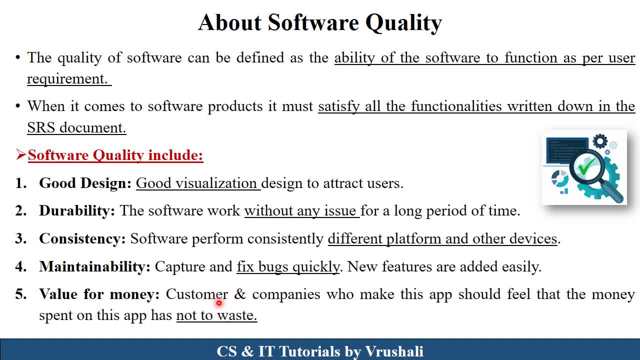 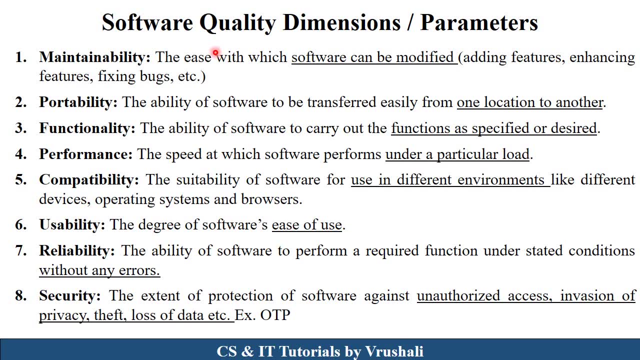 software and customer who give a requirement. both customer and companies are profitable not to waste a money here. this is called as value for money. so basically by considering all this attribute your software quality is decided. now the next topic is software quality: dimensions and parameters in software engineering. 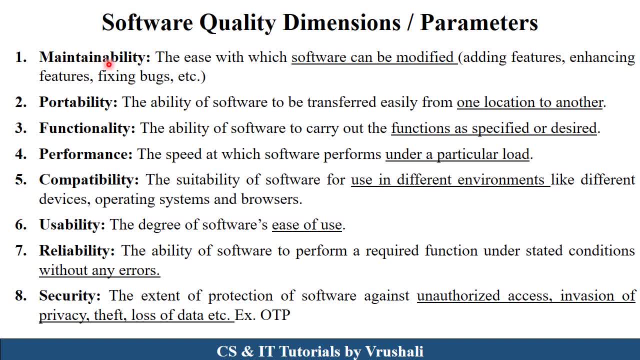 there are total eight dimensions. the first one is a maintainability. means when you develop a particular software in this way that can be easily modified. means you can easily add new features, new versions of particular product, and you can also fix or solve all the bugs and errors quickly. 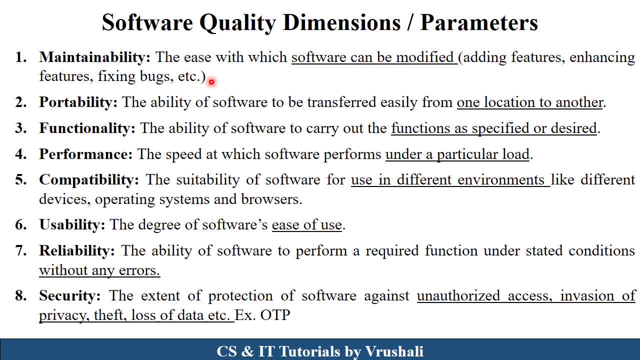 the best example is see. there are some applications like whatsapp, flip cards, and there are new versions are available each time. right, they provide a new features in this version, so this is called as maintainability. next one is a portability means your software can be transferred easily from one location to another or one device to another device. 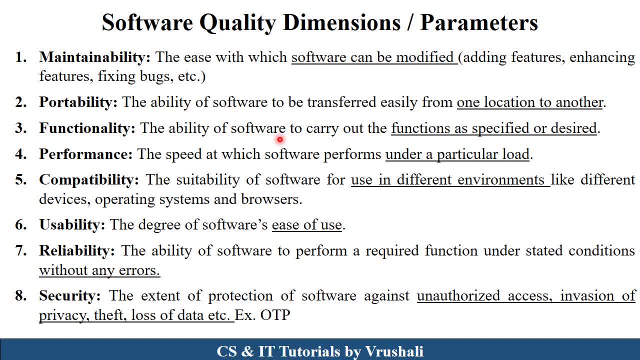 next one is a functionality. means your software fulfill all the need or functionality that exactly customer want. next one is a performance: means your software give a accurate result within a time. suppose a particular website or particular application used by the multiple users at the same time means they handle a load of that particular application. this is called as good. 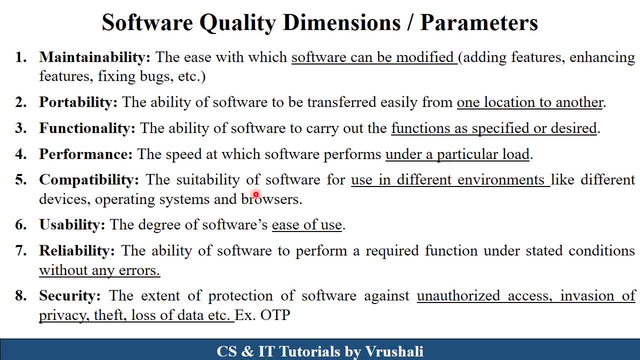 performance. next one is a compatibility means your software is suitable for use in other different environments, like different devices, different versions of operating system and different browsers. next one is a usability means your software is easy to use in different environments or that will be used by other literate or non-literate people as per their requirements. 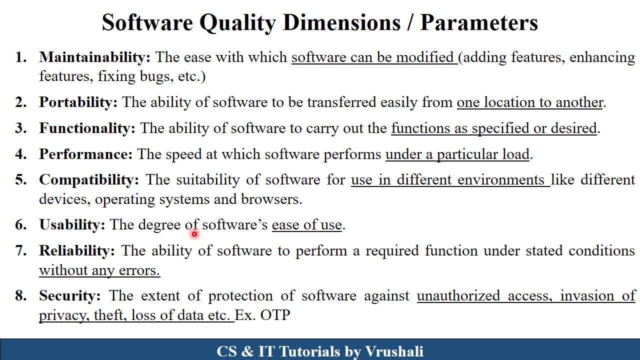 for example, there are some banking application that will be easily provide all the features which is necessary for banking users. the next example is online shopping application, so that will be also easy to use. so this is called as good usability. next one is a reliability means your software is work without any errors or without any bugs. means the software perform all tech applications. 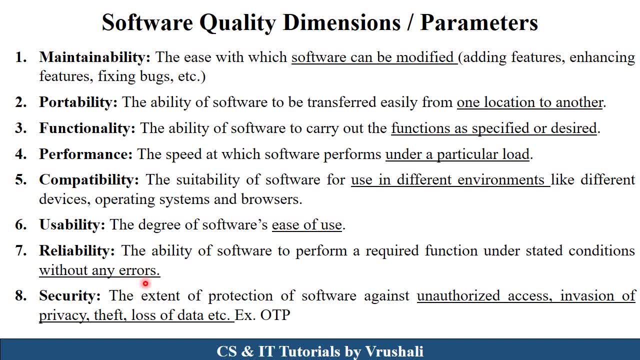 into the software without any errors. next one is reliability: means your software is work without any hours or without any perk. means you can 东タイ перminator, alian amsasp, or without any bugs, until face down from the first rapid check. The FTC does no work, So you just need a high power to authorization or a powerful battery of later drives. 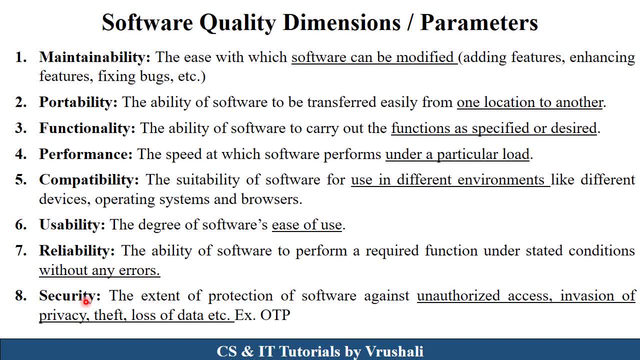 means they have a good reliability. and last one is a security means your software provide a protection against unauthorized access of users, then loss of data and privacy towards a system. the best example is there is otp, that is one time password, then two-way verification is there. they provide security towards your system. so this, all dimensions, are necessary. 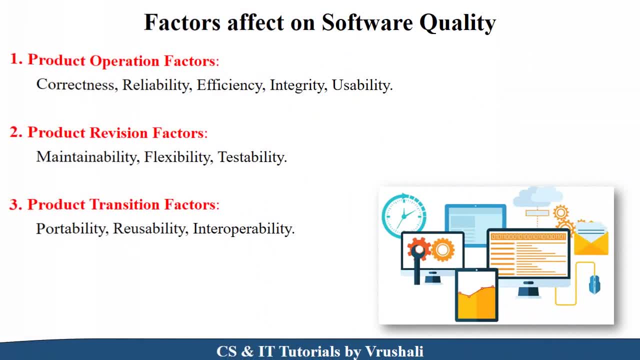 for deciding the quality of software. now the next topic is factors affect on software quality. this factors have divided into the three types, like product operation factors, product revision factors and product transition factors. first we understand about product operation factors. see, when you develop particular software in this way, they will give correct and accurate. 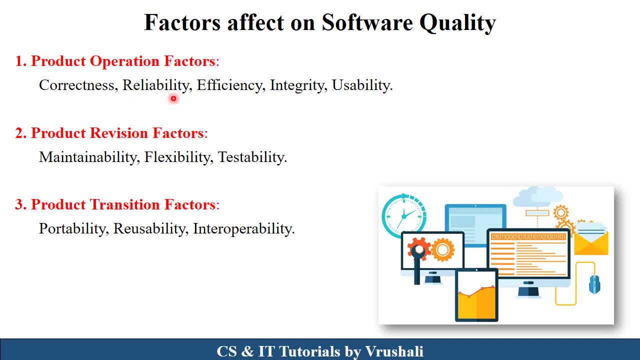 result they we have good reliability. they can easily solve the all reportf of the software, especially illiterate software, so we can solve for good ситуational task and also they provideGOGOTS and lost time and they provide stimulant and or errors. they have a efficient performance. integrity means valid data. 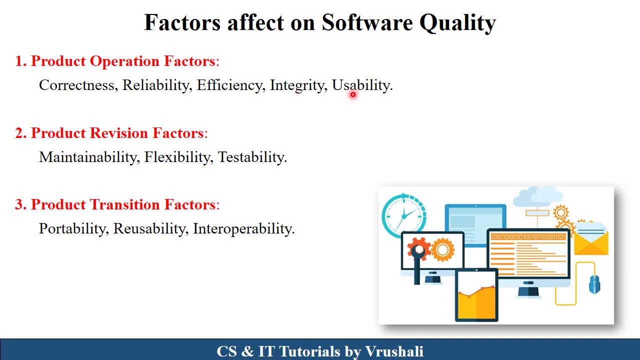 valid information have stored and easy to use by all the other users. so by considering all this product operation factors, consider the quality of your software. next one is a product revision factors. that is, maintainability means you can easily add new features in particular product that will be good. 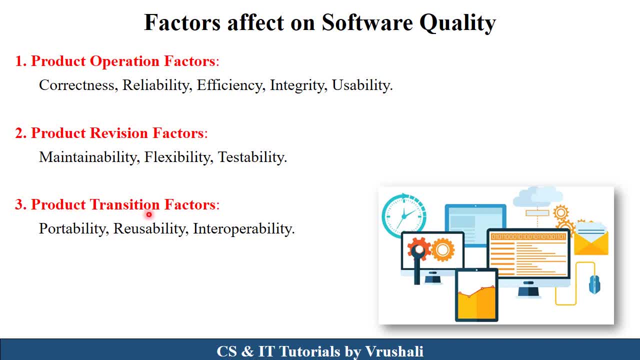 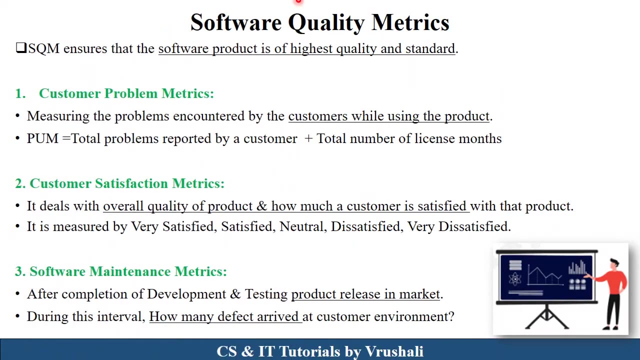 flexibility and testability. next one is a product. transition factors means the portability- your product is easily transferred from one device to another device- and good reusability. interoperability means every manipulations, every operations can be performed easily. so by considering all these factors, your software quality have decided. now the next topic is software quality matrix. 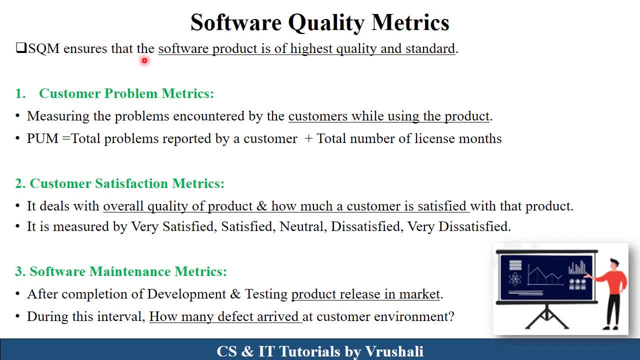 basically, this software quality matrix is based on the performance. of the software quality matrix ensure that that your software is developed as per the high standard and highest quality. this matrix have divided into the three types, like customer problem matrix, customer satisfaction matrix and software maintenance matrix. first we understand. customer problem matrix means when you 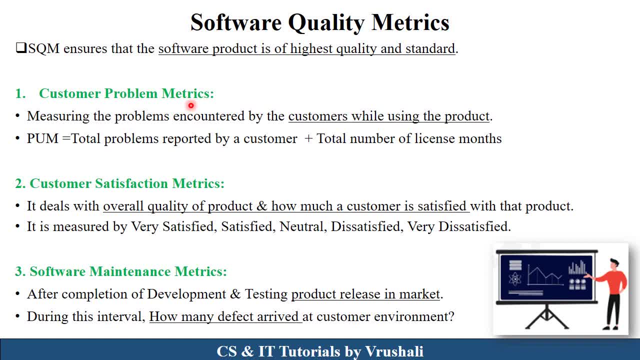 deploy a particular product or software in market. customer use a particular product. now, while customer using a particular product, there are some errors or problems are faced by the customer. so basically, this customer problem matrix measure all the problems encountered by the customer. they measure total problems reported by the customer. next one is a customer satisfaction. 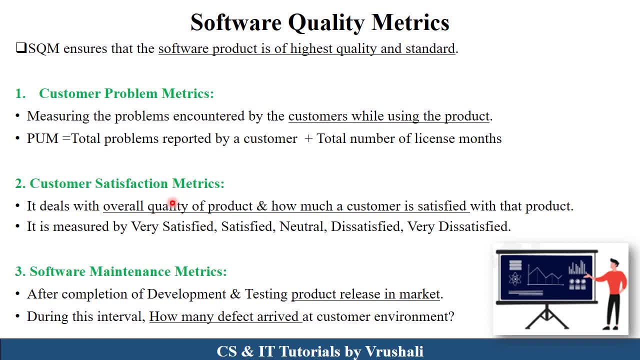 matrix. basically, after deploy product to the mat or to the particular informant or market, they give a feedback from the customer. so feedback can be given in rating format like three-star, four-star, five-star rating, or also it can be measured by very satisfied, satisfied, dissatisfied or very dissatisfied in 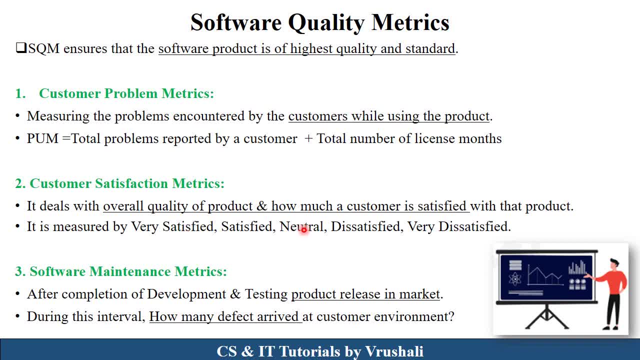 this particular format. generally, these metrics are used in every online shopping application like flipkart, amazon, myntra, in this way. next one is the software maintenance matrix. after completion of development and testing of particular product, your product release in market. in deployment phase of software development life cycle. now at customer environment. how many errors. 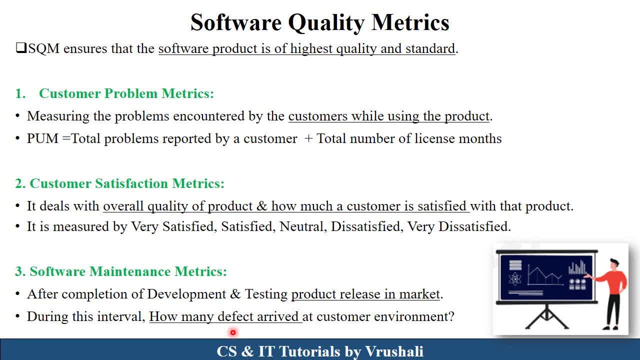 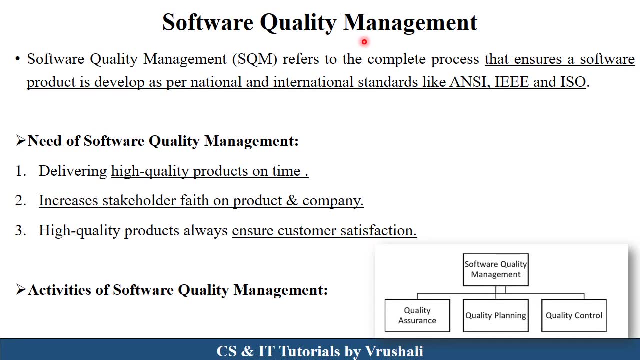 have arrived, how many defects are arrived. this can be calculated in software maintenance matrix. that's why this, all three metrics, are important, measuring the quality of software. now the next topic is software quality management. basically, this software quality management ensure that your software product is developed as per the national and international standards like ieee, iso standard or they also. 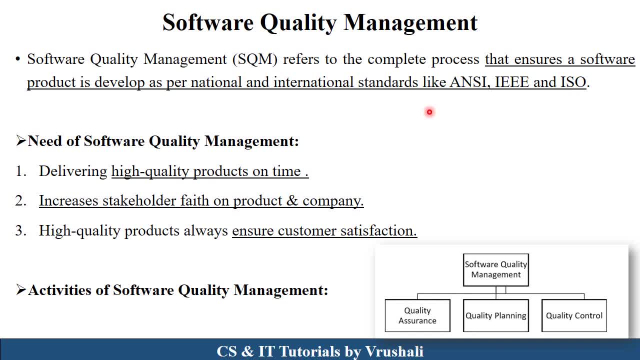 ensure that your product is developed as per your government or country roles. now what is the need of software quality management? this software quality management ensure that your product is delivered, that in high quality format or on time. they also increase the faith on particular product and particular company. basically, they ensure 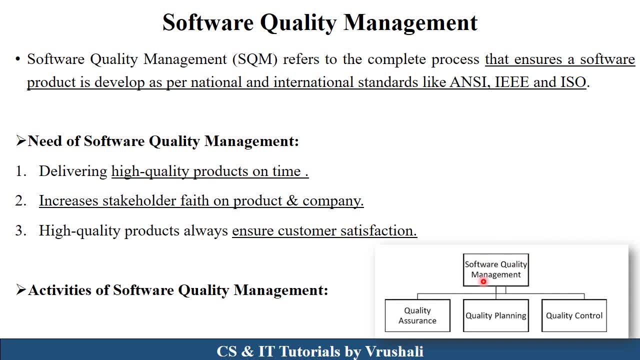 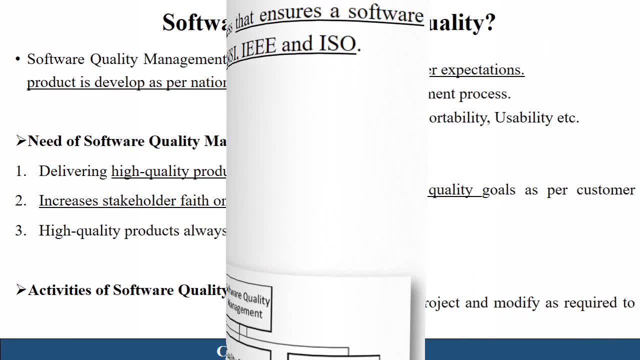 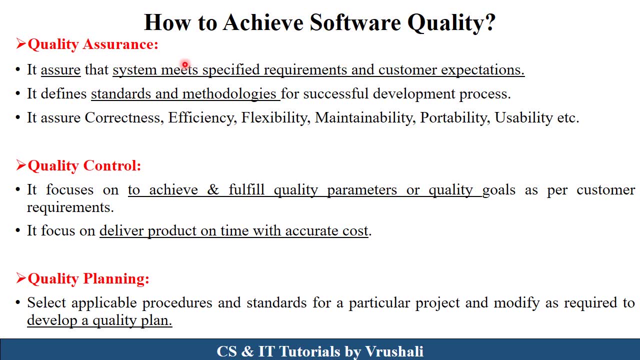 the customer satisfaction. now this software quality management having total three activities like quality assurance, quality planning and quality control, the next topic is how to achieve software quality. for that purpose we use three activities of software quality management. the first one is a quality assurance in quality assurance. here software quality manager give 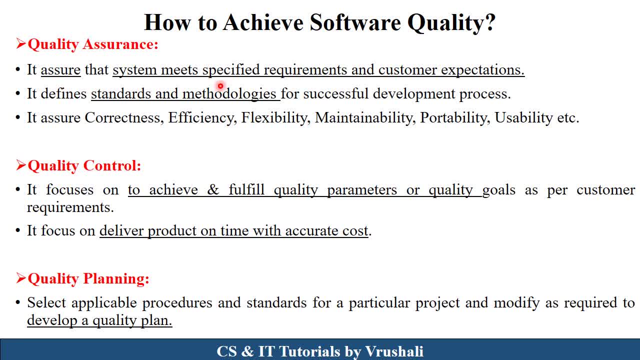 assurance, promise to the customer that they can deliver quality assurance to the customer, develop a particular software as per the customer requirement and customer expectation. for that purpose they define different standards, methodology and complete development plan. basically, they assure to the customer that is: correctness, efficiency, flexibility, maintainability, portability. 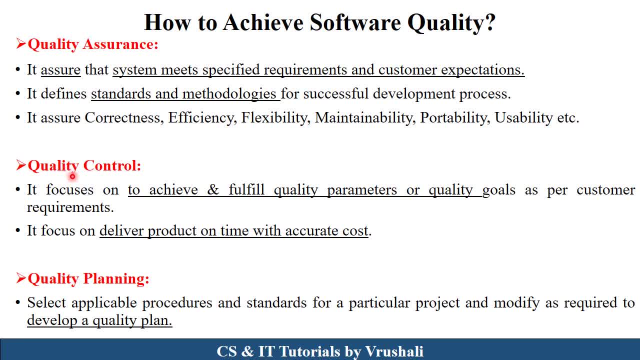 and usability of particular software. now the next one is a quality control. so quality control focus on actual development of particular software. they focus on actual quality goals and customer requirement fulfillness regarding a particular product. in quality assurance they just give a assurance, but in quality control they fulfill those assurance. they mainly focus on your 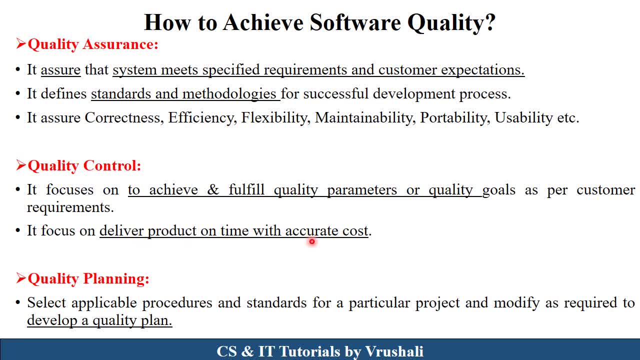 product delivered on time with accurate cost. in next session we will discuss about quality assurance versus quality control. this is one of the most important topic as per your exam point of view. and the last activity is quality planning. here, software quality manager develop a complete quality plan or development plan regarding a particular product. for that purpose, they use different. 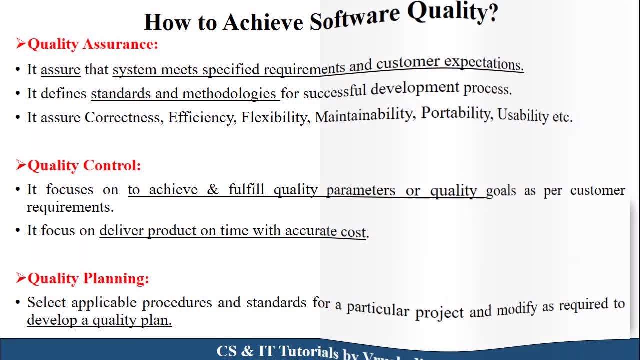 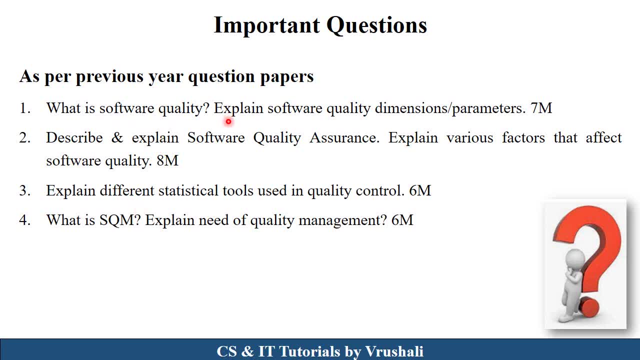 procedures, standards and methodologies. now, as per your previous year question paper, these questions are important, like: what is software quality and their dimensions? for seven marks, describe and explain software quality assurance and their factors. for eight marks, then, different statistical tools used in quality control. for six marks, and what is sqm? explain. 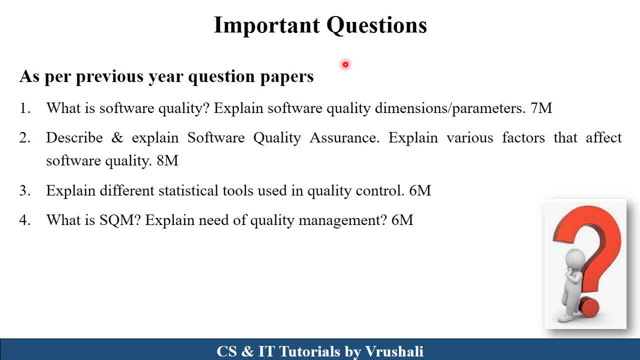 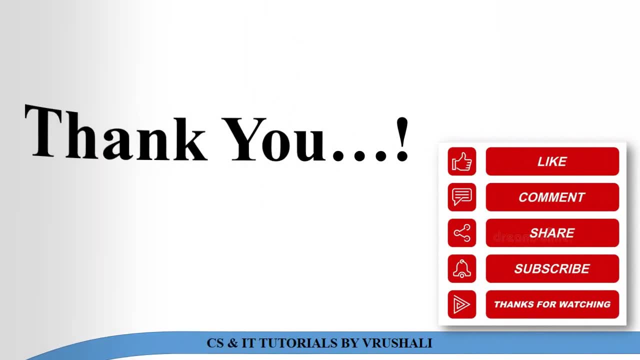 need of quality management for six marks. so you have to prepare basically complete software quality topic as per your syllabus point of view. so this is all about software quality. thank you, keep learning. 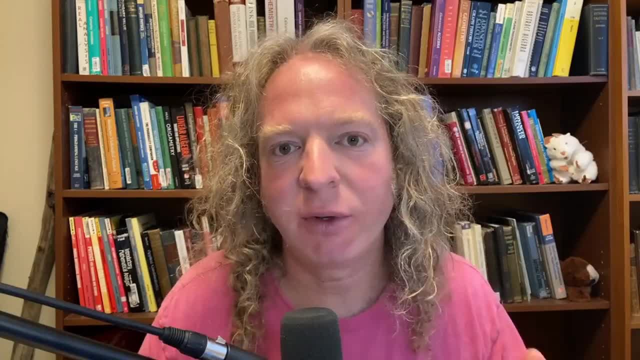 Hi, in this video I'm going to be reading an email I received from a viewer and doing my best to answer it. As always, if you have any advice for this person, please leave a 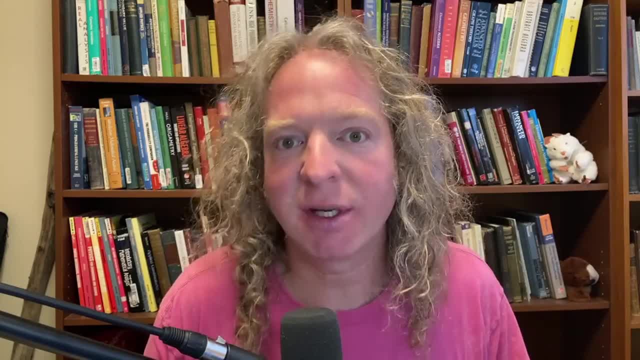 comment in the comment section below. Remember, people read the comments and so every time 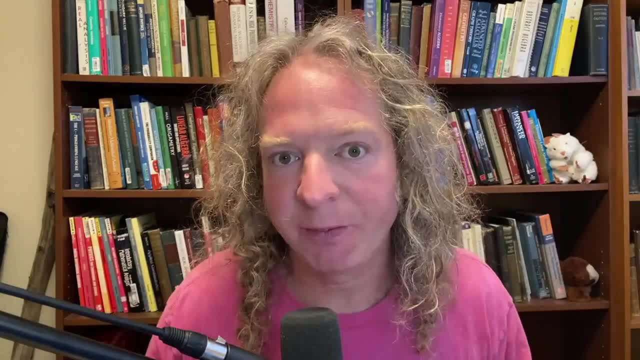 you leave a constructive comment, it really helps other people. Let's go ahead and open 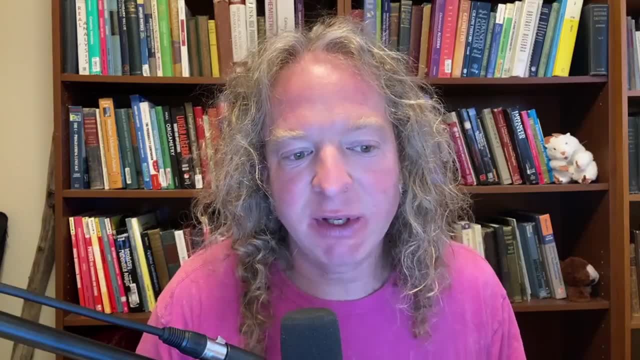 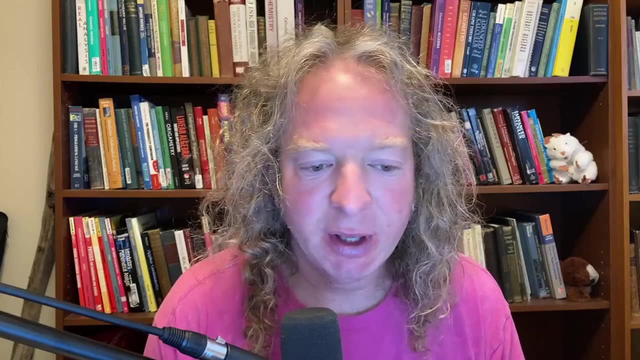 up the email here. And the person's name is Sudeshna and the subject is Tips on Problem Solving. Hello, I am Sudeshna. I am 17 years old and I recently completed my high school. 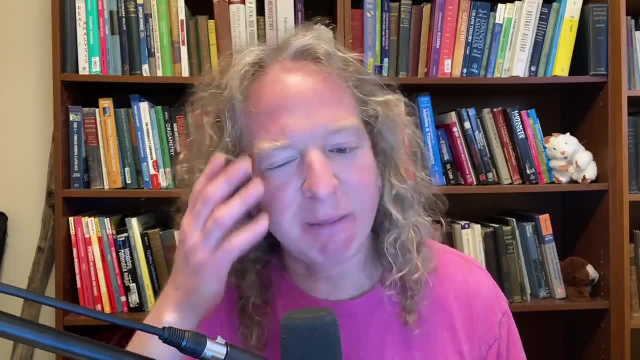 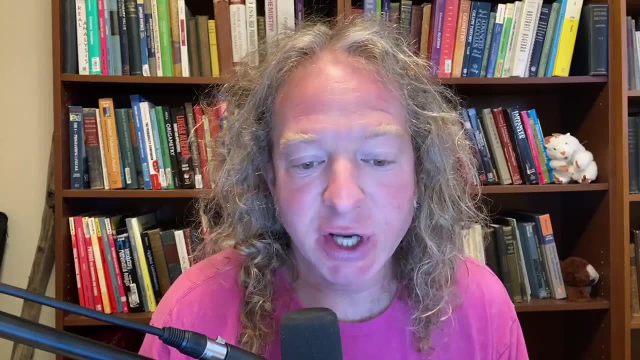 I am studying maths on my own. While I feel confident that my basic high school math, I am attempting to move to advanced high school maths. Currently, I am studying number theory from Elementary Number Theory by David M. Burton. Though I do not lack necessary resources, 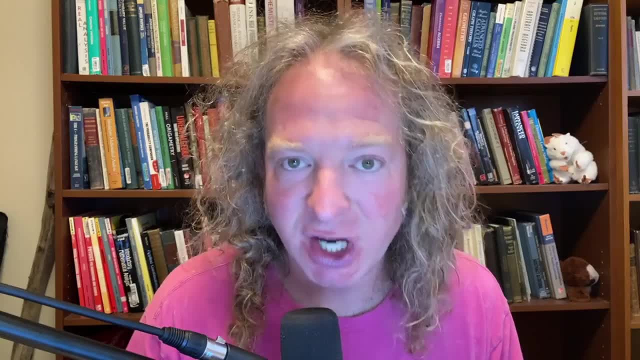 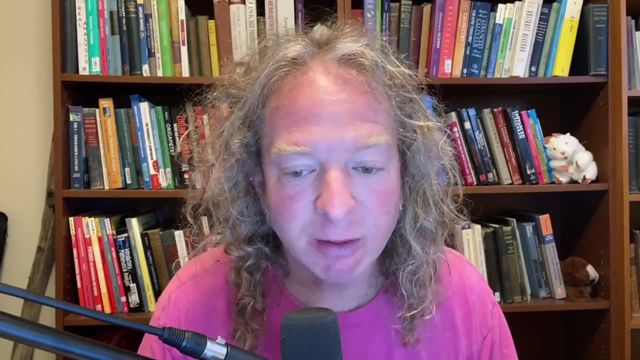 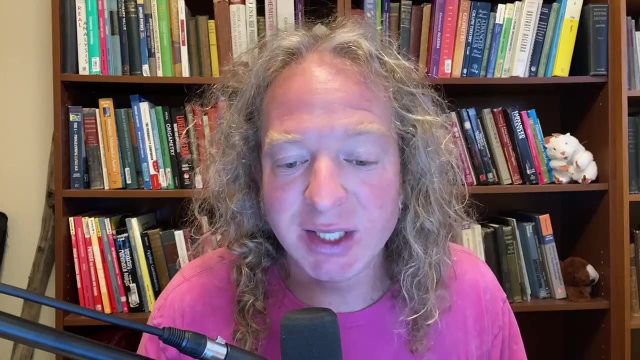 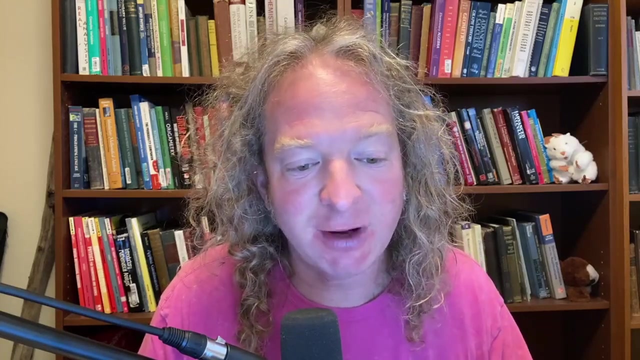 which are easily available through books and YouTube, I find myself stuck when solving problems. I feel I have a good grasp on my common sense and I am able to solve problems on a particular topic, but when I move towards the problems, I get stuck with one problem and spend hours on it, which is in no way helping me improve. However, when I see the solution to the problem, I immediately can know why is the particular solution the solution so that the problem and at times I do find myself trying to think of a different way